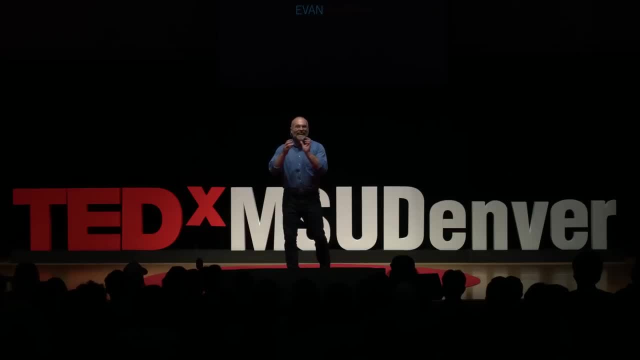 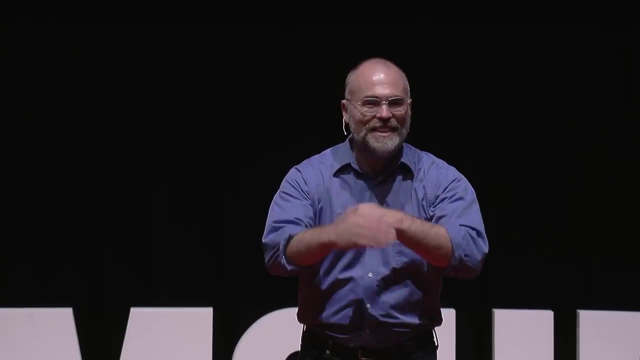 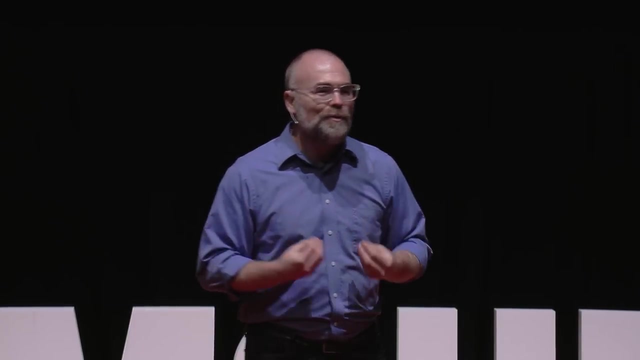 I'm glad I chose the latter and I signed in silence that phrase to my clarinetist: you continue with this. And not only did I get back a sound which was more haunting and wondrous than I could have imagined, but I also got a sound which was more haunting and wondrous than I could have. 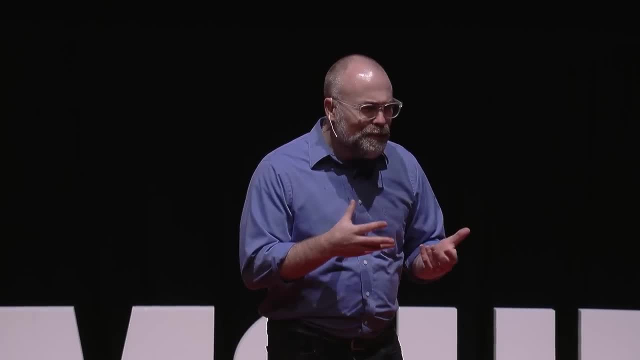 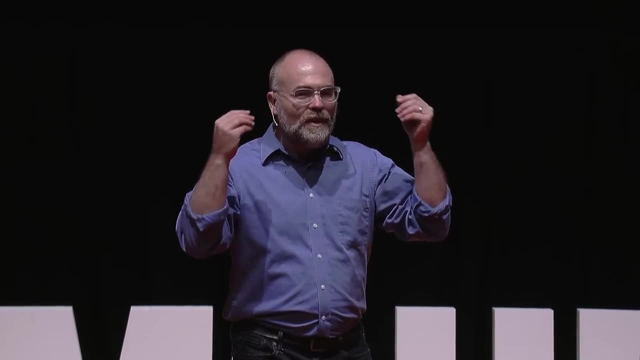 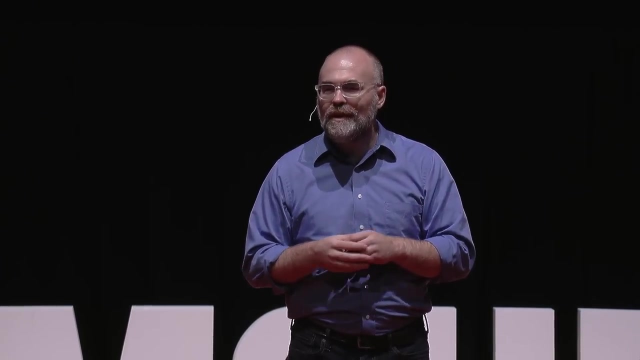 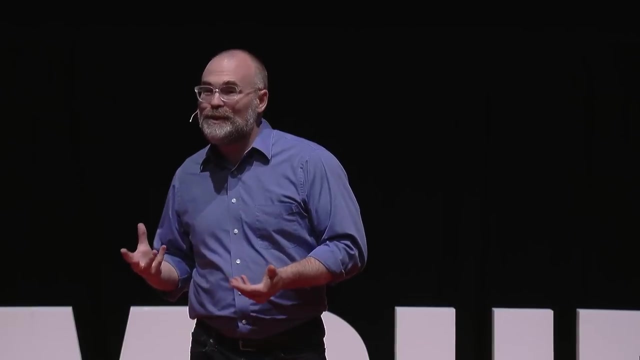 composed one that sounded more like a bamboo flute than a clarinet. I also received an insight into what it takes to be a leader in education in the 21st century. So today I want to talk about how I arrived at that moment on that show to say yes to the surprise. 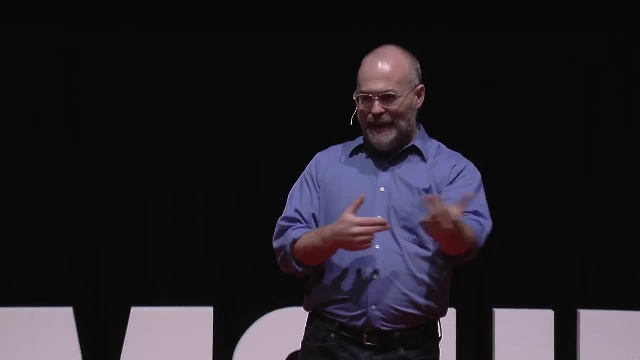 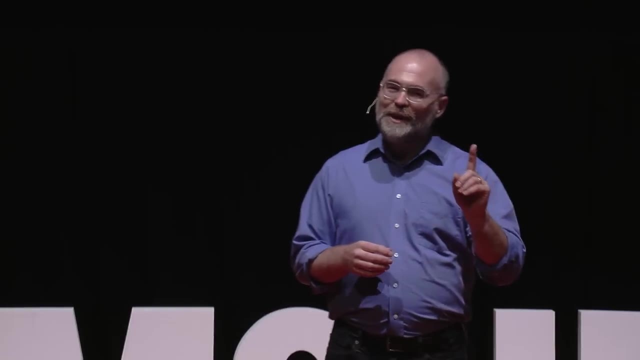 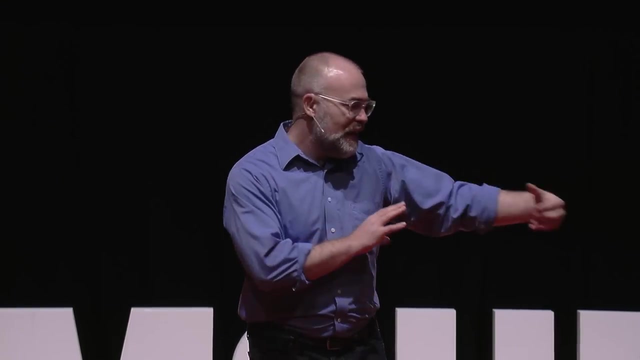 and why my journey even matters to the field of education And what there is to do, And we're going to close with a group exercise. But before we get there, how did I get to that moment to say yes to such a shocking surprise? What you don't know is that I 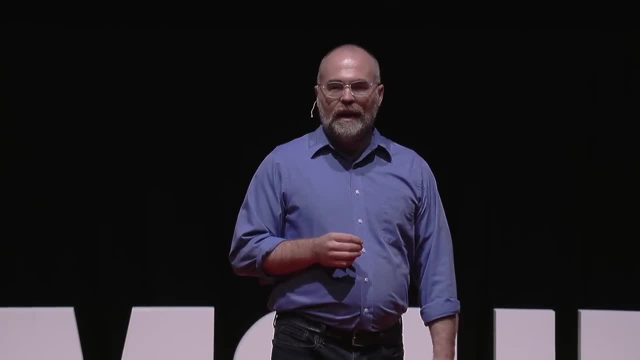 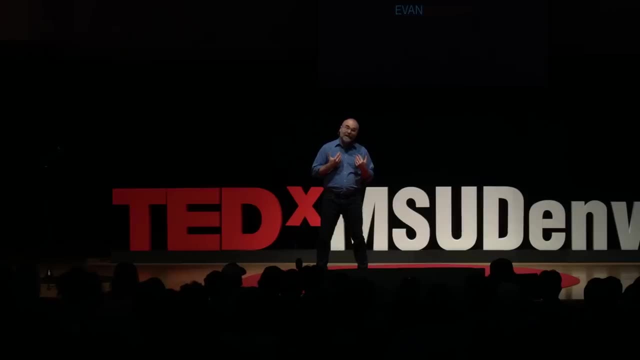 started piano at the age of four and in one of my very first public recitals I actually ran off the stage in tears because I had made a mistake and not played what was on the page. And I was making the same mistake over and over again because I really didn't know what I was doing when. 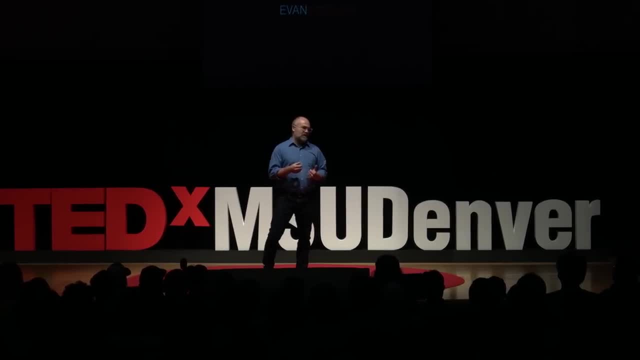 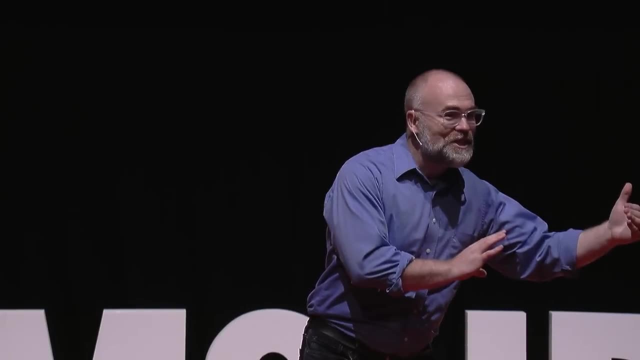 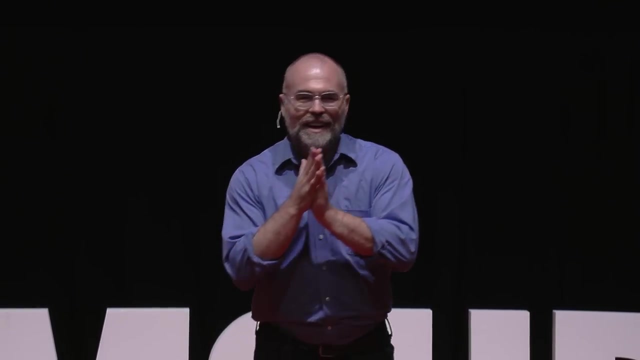 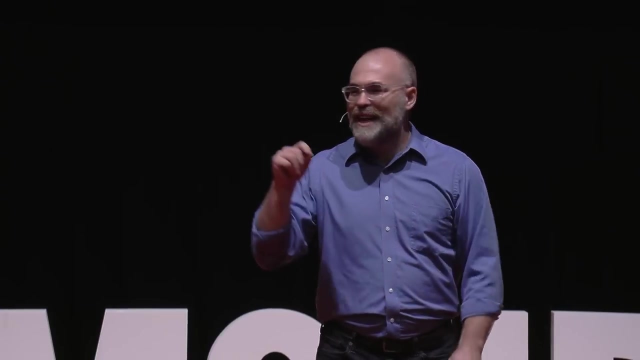 I was playing. You see, in many ways I was the product of a very traditional music education, one that prioritized perfection over innovation, One that championed competition over collaboration. But along the way, I had several mentors and educators who poured into me, And they enabled me to take risks and to make creative choices selected themselves. 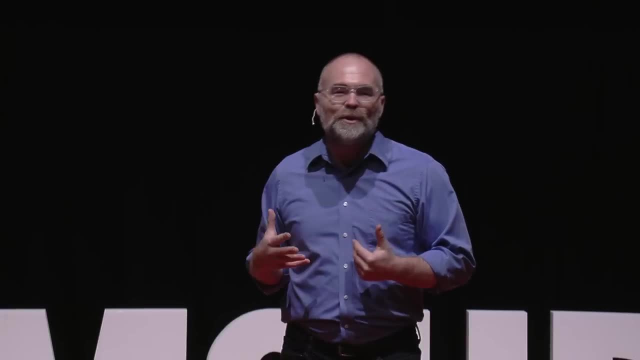 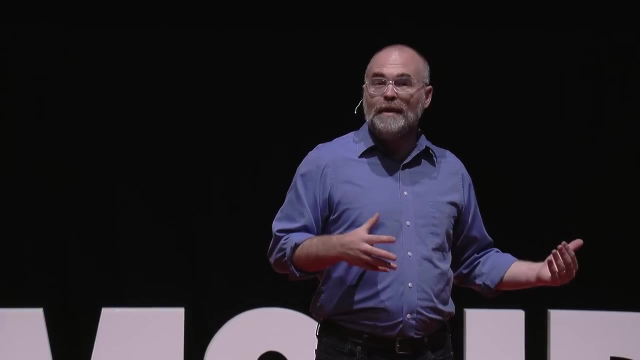 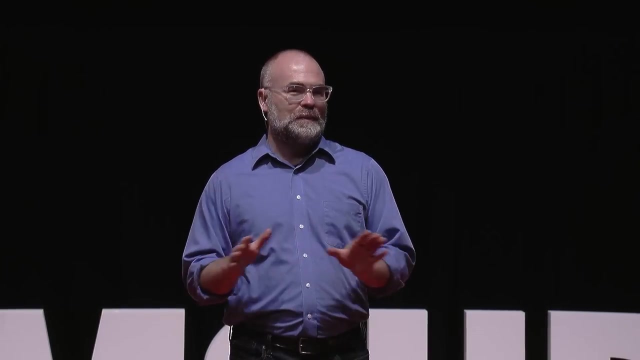 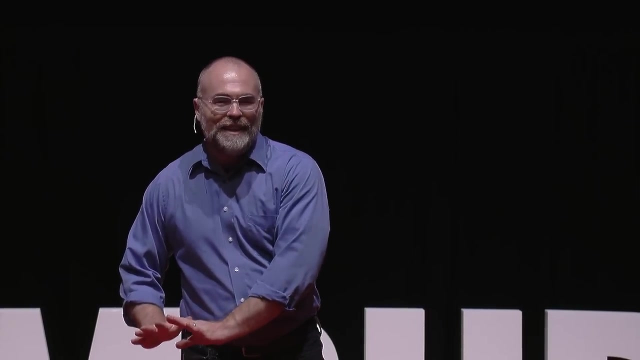 whether it was improvising on a blues solo or creating a piece for a concert, or even stepping out on the stage with them as educators and improvising an entire concert with nothing on the page. But why does my journey from timid beginner to confident professional even matter to the field of education? 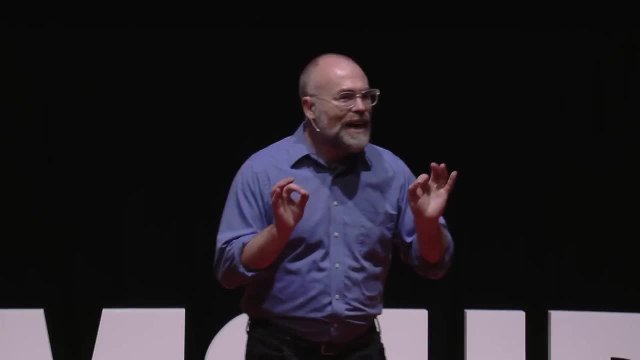 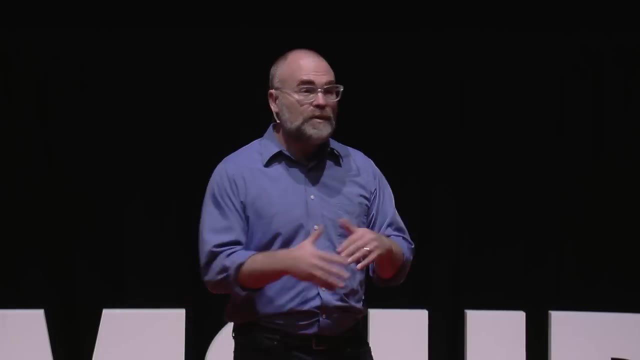 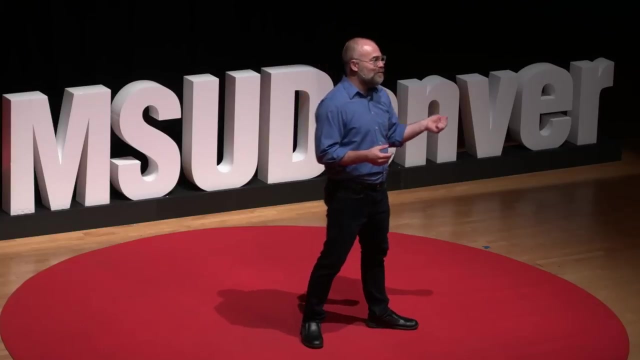 Well, we are entering one of the most complex, unpredictable and rapidly changing landscapes we've ever seen. as a species, As a modern civilization, we've turned the page several times, from the agricultural to the industrial, to the information age, and we are now in what author Daniel Pink calls the conceptual era. 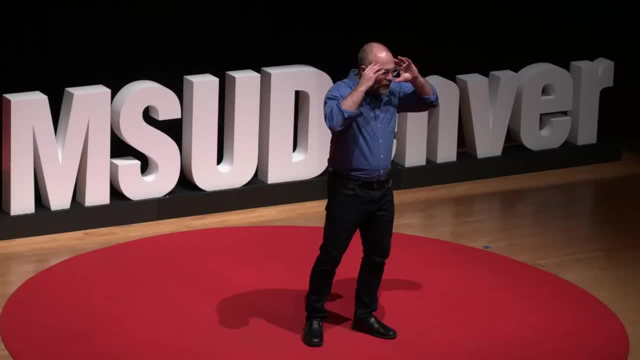 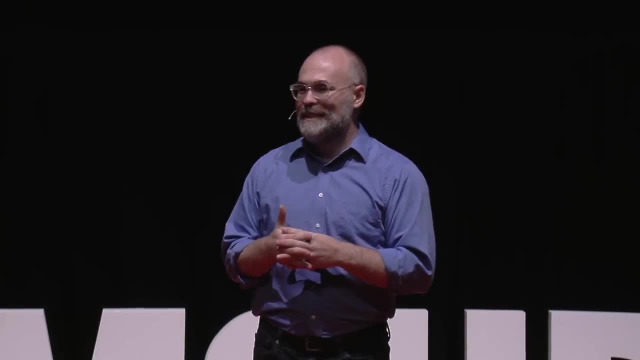 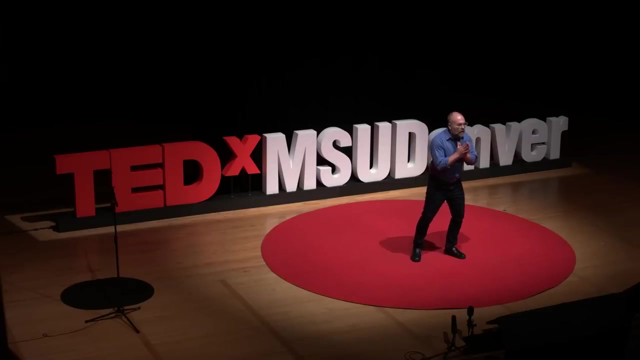 And in this era- we are in a time of a modern civilization- We are in a time of a modern civilization- Those concepts of empathy and play and symphonic-like collaboration are what will make the difference in such a rapidly changing environment. The World Economic Forum says that 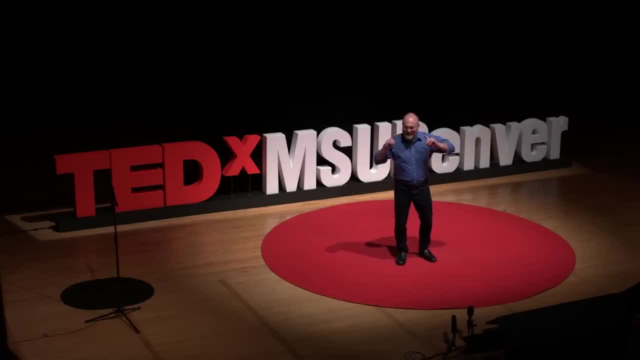 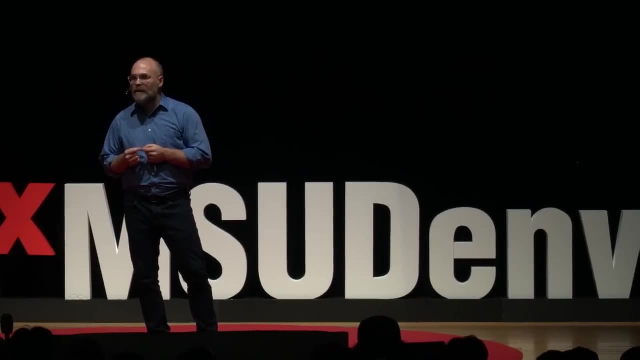 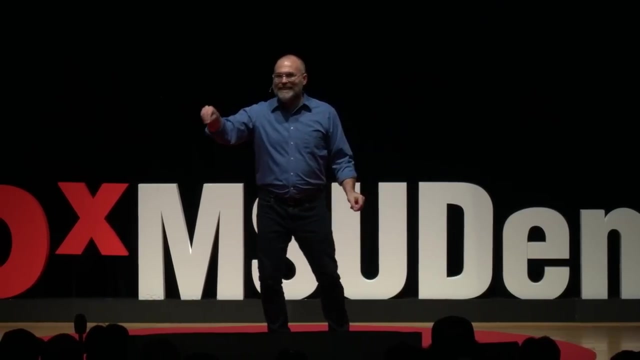 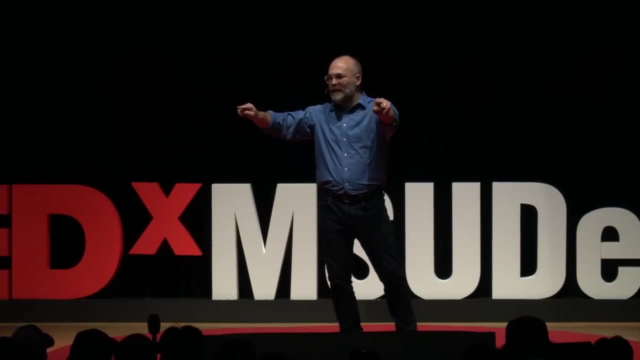 those soft skills of active listening, of creative collaboration, of complex problem solving, of creativity, of creativity are what will make the difference and will set those who are ready up for success in this new era. But if that's the case, if this is the future we're facing, 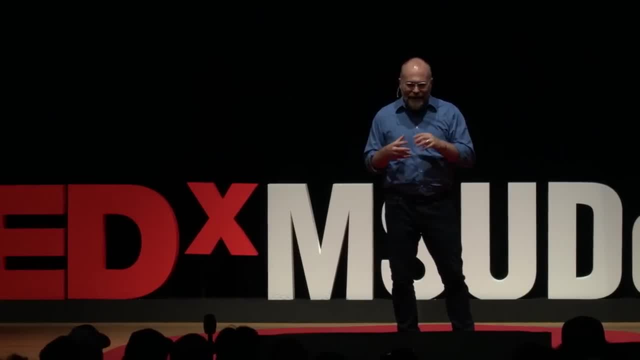 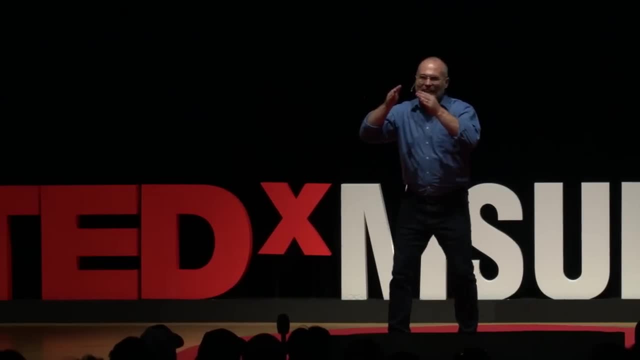 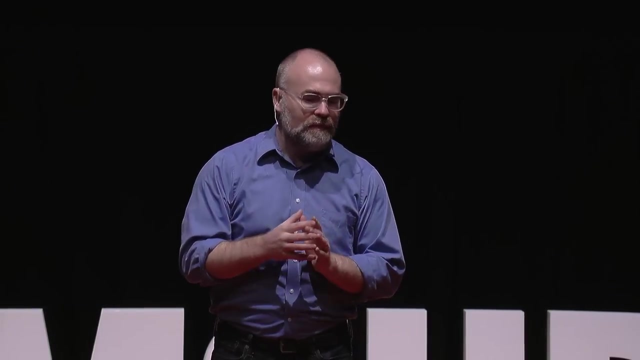 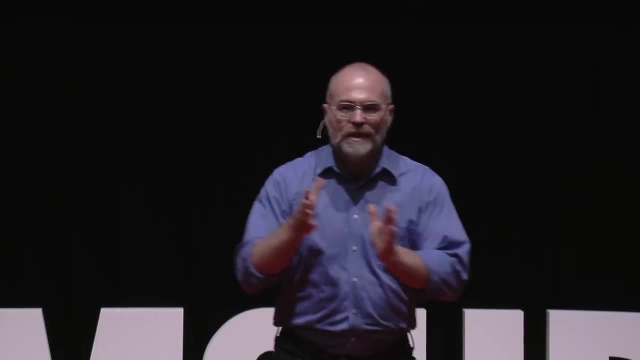 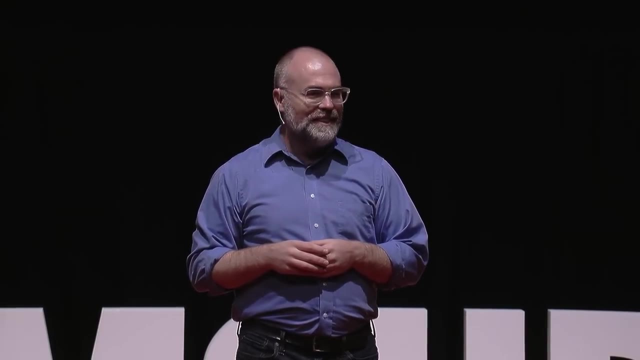 Why do we still proceed as if narrow specialization and skill building is the ultimate benchmark? Why do we go forward with these old models into this new future? Why do we go forward with these old models into this new future? Well, for starters, creativity is messy. 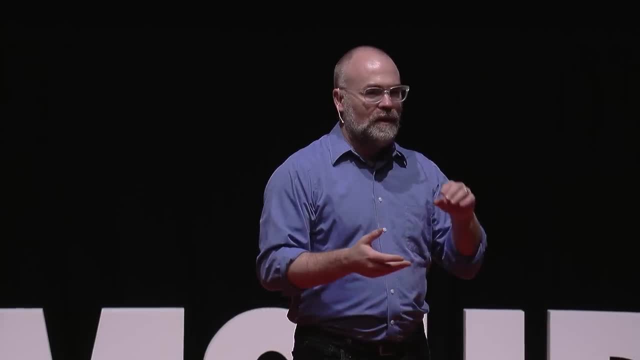 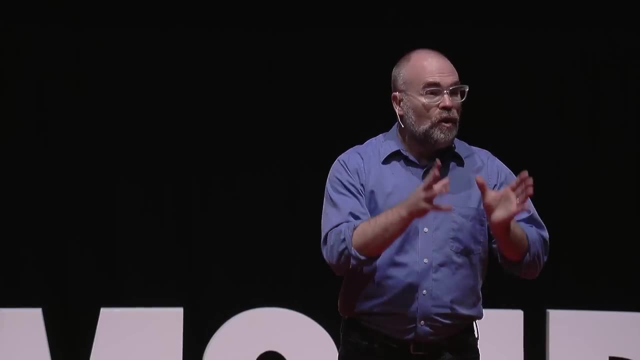 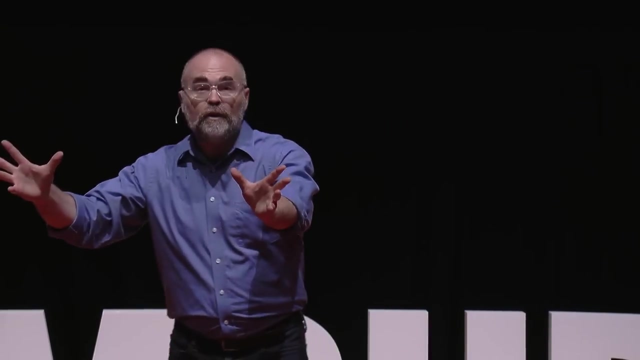 It's not easily assessed, measured, graded, tested. But for those leaders in education who are ready to rise to the challenge, who are ready to rise to the challenge, are ready to face their challenges to step into this new future, are ready to go beyond outcomes into adventure, are ready to 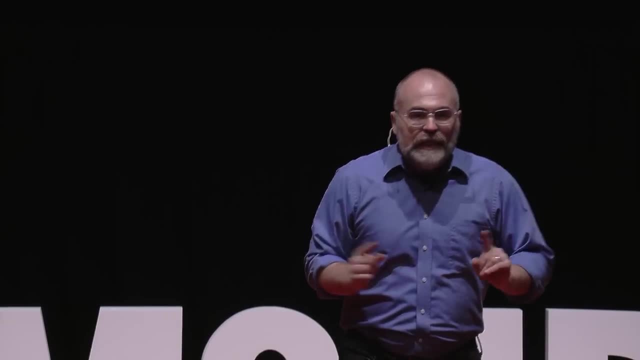 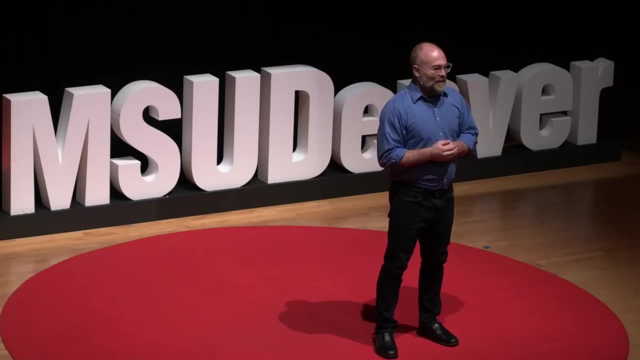 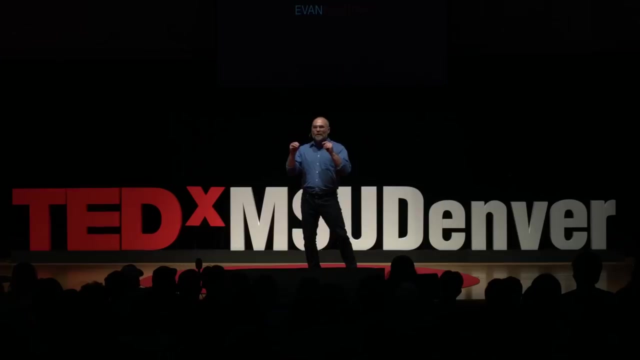 push past those old models, are ready to lead those they mentor into a liquid mindset, into resiliency, are ready to lead those they teach to experience the power of play. If they are ready to do that, they are ready to lead those they teach into this new era. So the call is clear. 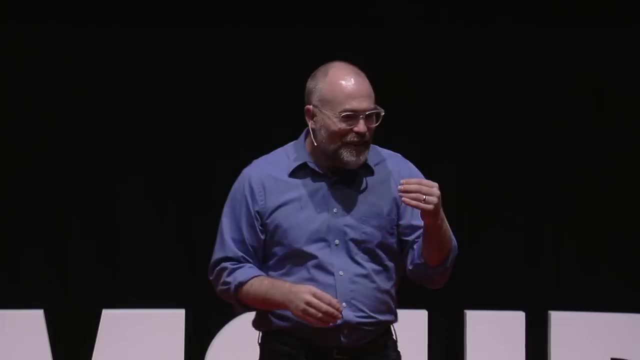 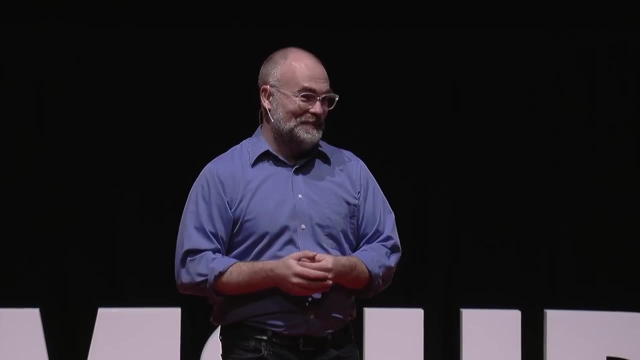 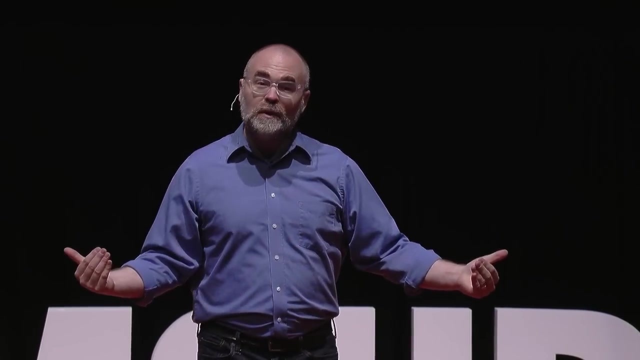 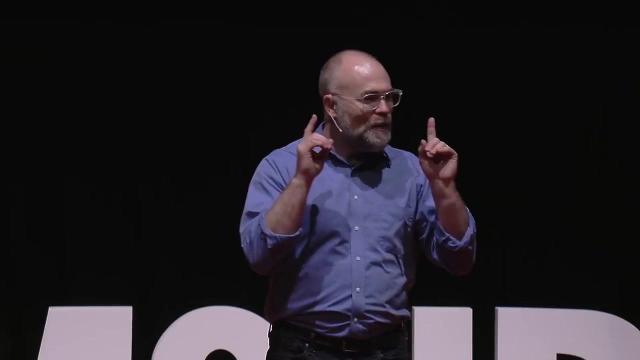 What is there to do? Simply this: create scenarios in which you, as a leader, do not know the outcome. legitimately, Put yourself in scenarios where those you're mentoring have to step into the unknown with you and make that discovery possible Together. But I don't want to just talk about this today. I want to put it into practice. 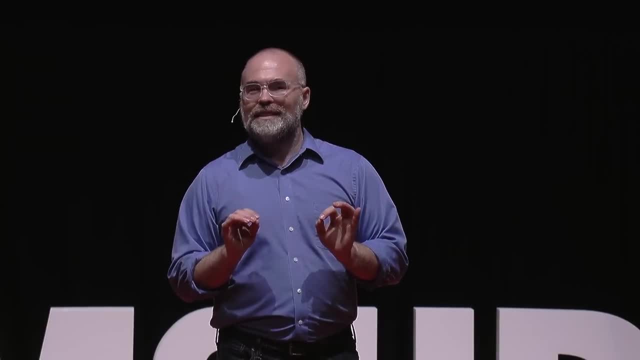 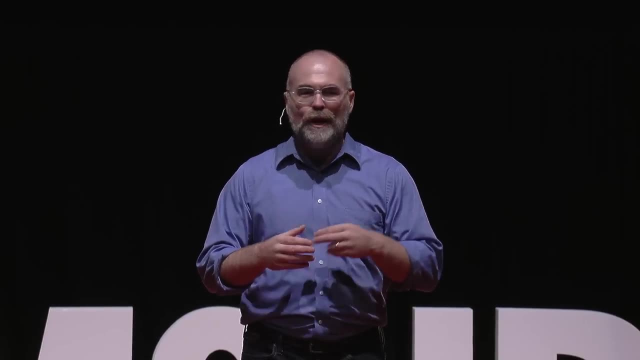 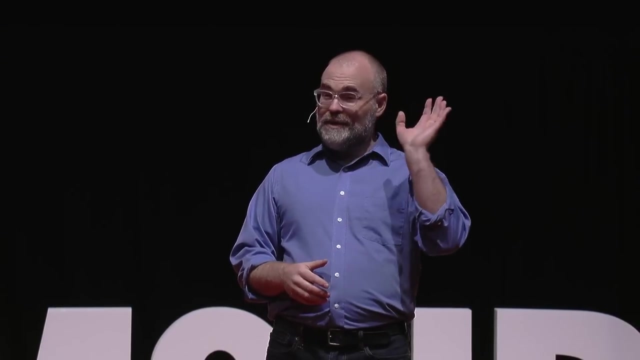 So I'm going to invite us to close in a group exercise and we're going to find the magic in this moment. We're going to make something amazing together. We're going to compose instantly and create a piece. And if you're saying to yourself, I am not musical. 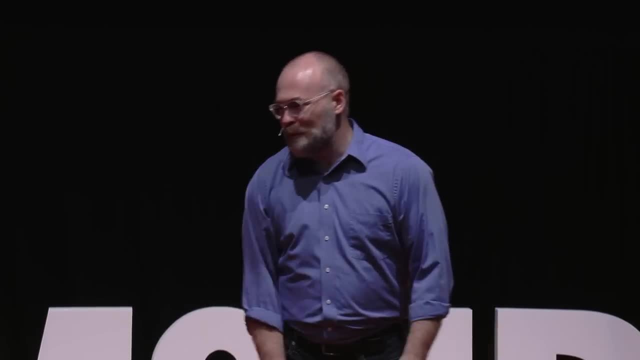 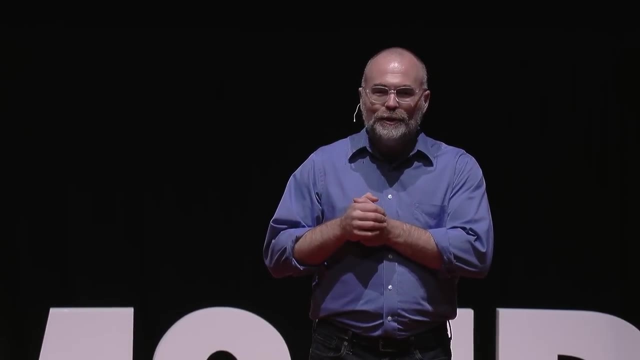 I am a Hebrean being to us. We're singing Pga buried, Never fear, We are just going to make a joyful noise here together and have some fun. And to help us I have invited a friend and colleague to join us. professor Mark Harris is. 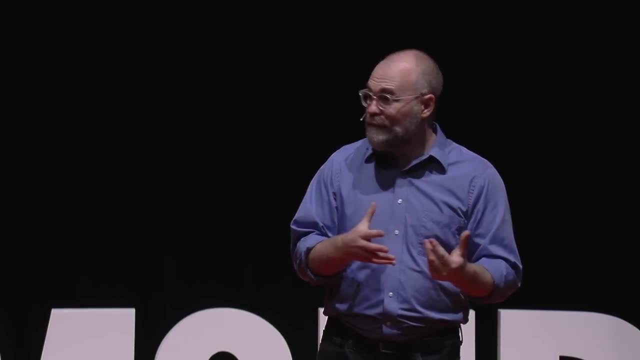 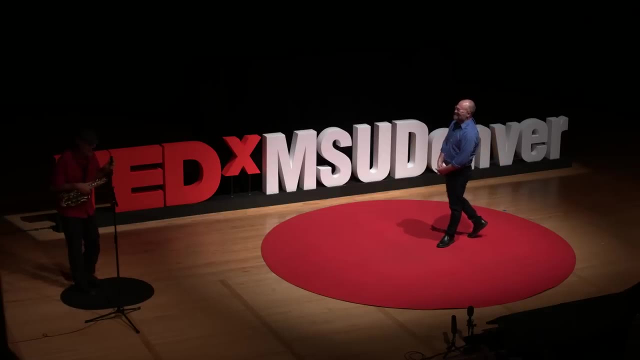 here on faculty at metro Metro. So would you help me in welcoming Mark to the stage Now? don't think you're too far behind because we haven't rehearsed what we're about to sing. I don't think we're hide or not. we've been able to develop fry. 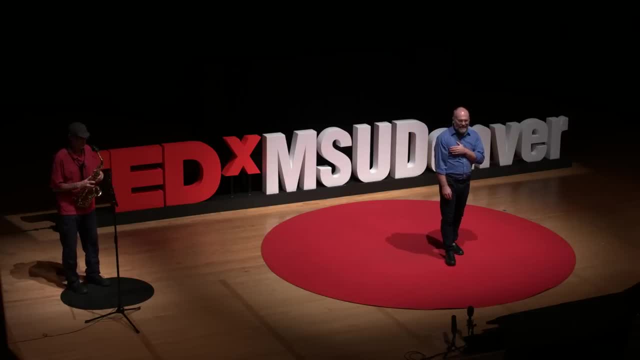 Now. I really want to thank Mark Harris and his team and his ability to answer questions And virtually the team will not have enough time to yet Melissa is one of our people And I want to thank herself and our four colleagues on stage for a chance. 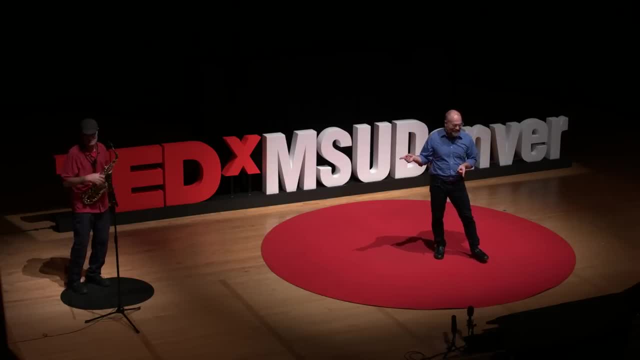 you're too far behind because we haven't rehearsed what we're about to do. So I want to create something together with you, and the way we're going to do this is: I'm going to embrace risk by stepping out as a leader and asking you to make a creative choice in response. right, So I'll give. 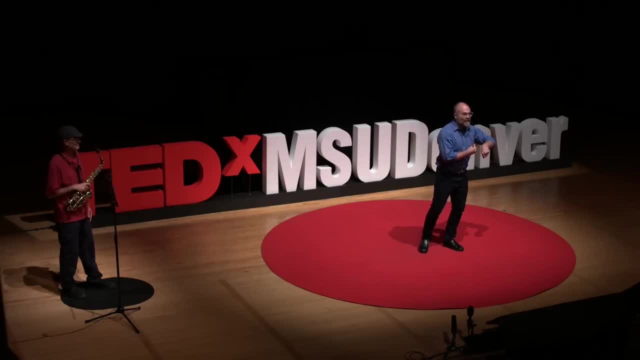 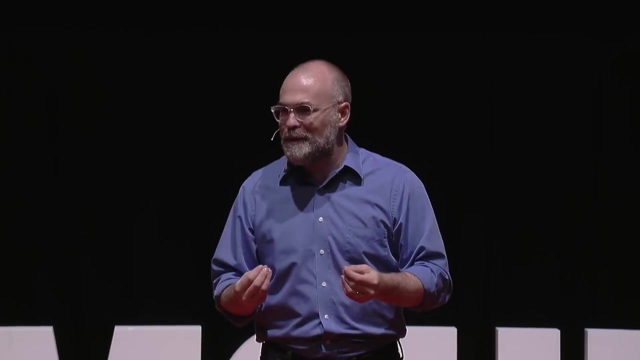 a structure and you can provide a content in response. I'll give a sign and you can give back some type of sound, all right, And each sign has a definite meaning. but feel free to reinterpret that sign every time I give it to you. So we've already learned one. I'll give this one to you for. 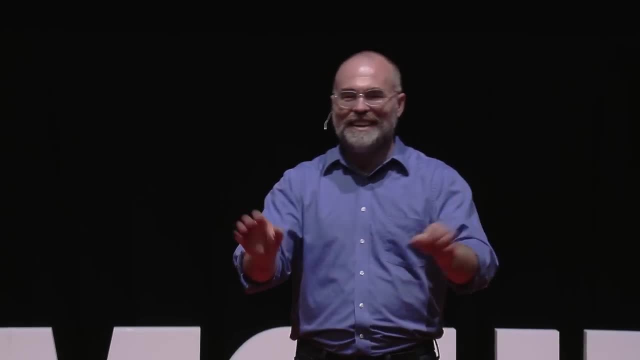 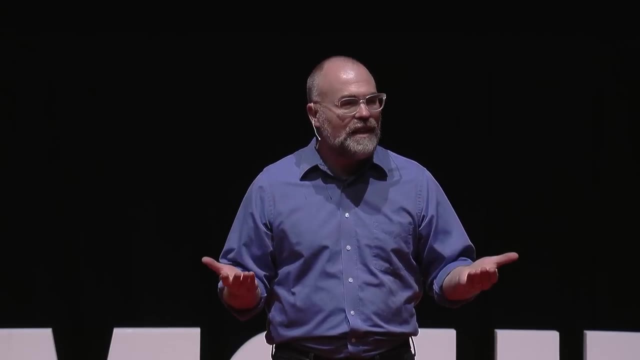 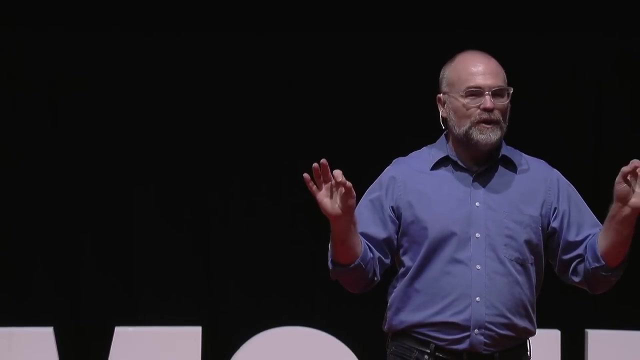 free. This is continue right, It's not traveling, It's continue okay. And we're going to learn three. It's hit, sustain and synchronize. Hit, sustain and synchronize. So let's practice The first one. a hit is a short, sharp sound right On my cue, Something maybe like this: 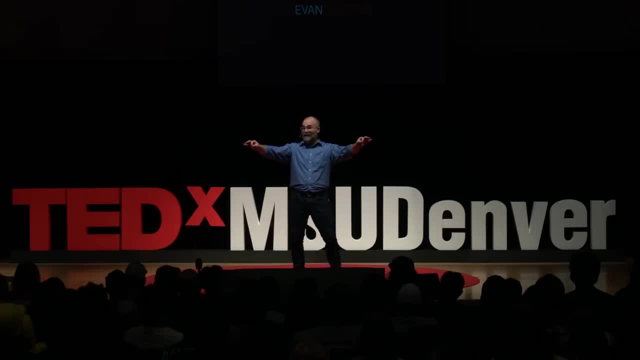 You ready? Even shorter, Great. And each time you can think of a new short sound Ready. Okay, we're getting warmed up. all right, Here's the exact opposite. right, It's a sustain. Pick one long tone. 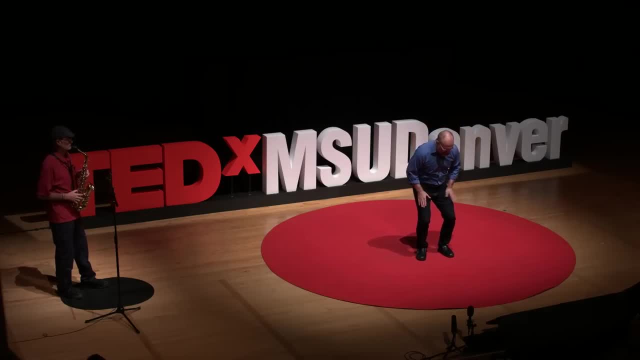 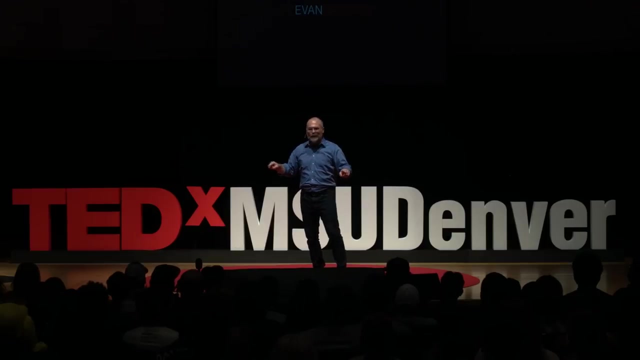 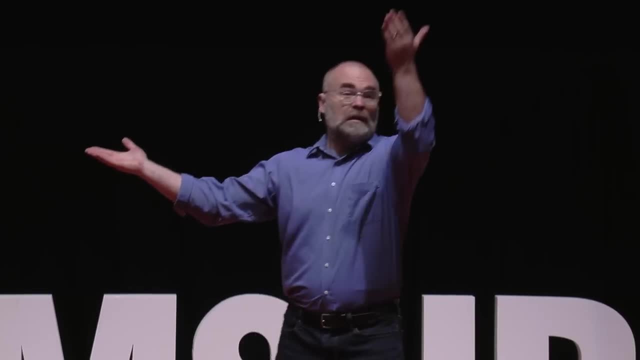 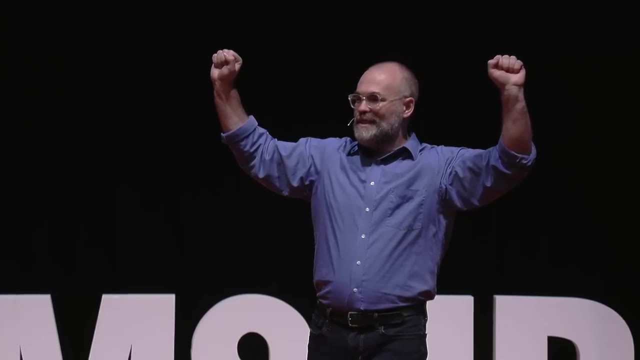 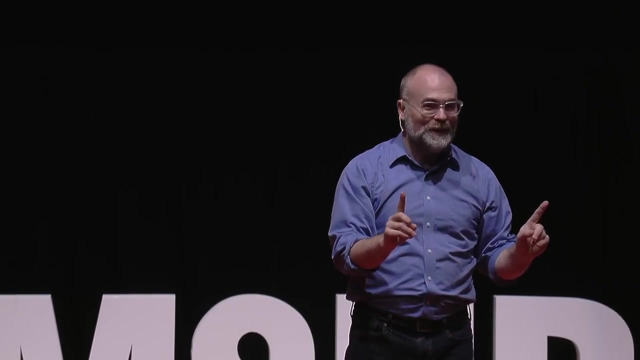 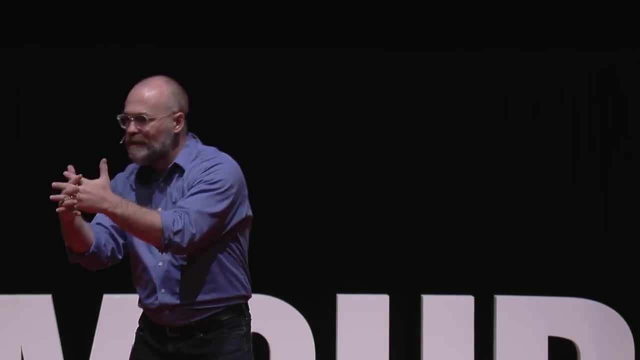 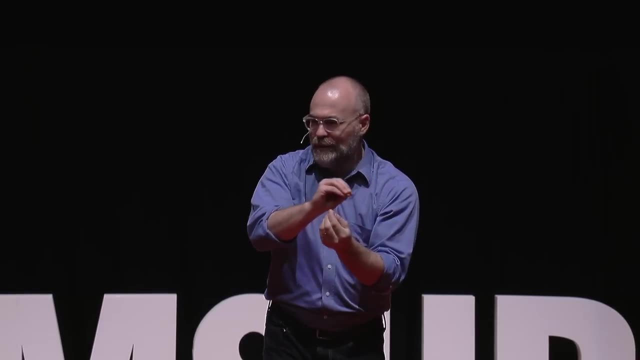 right. So, whatever we're doing in the moment when I give you this sign, start listening to those around you and try to merge your sound with your neighbor's right. It's a process of discussion, It's a process of sharing, It's a process of learning, It's a process of understanding. 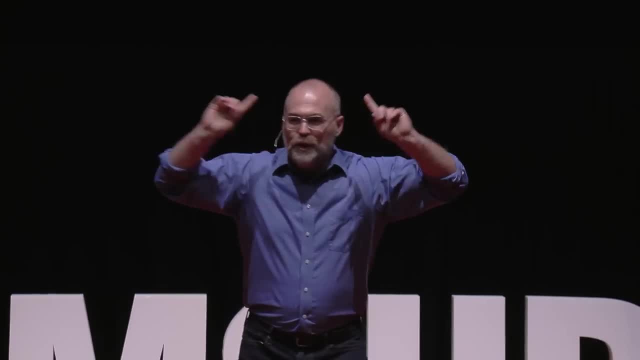 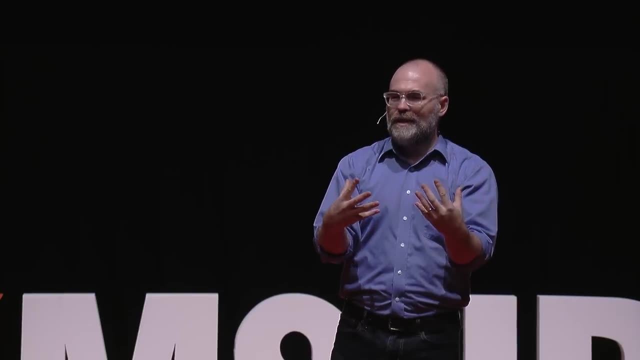 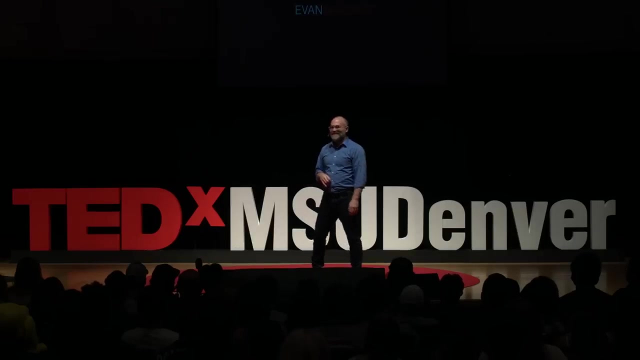 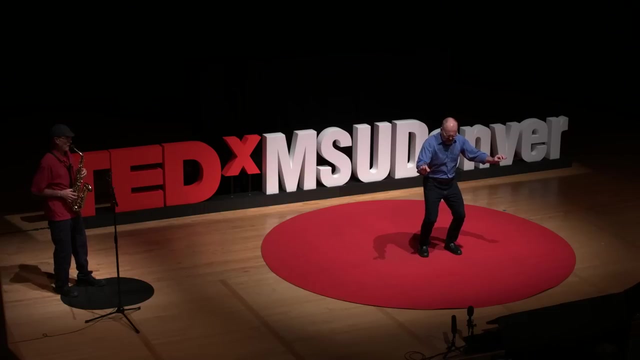 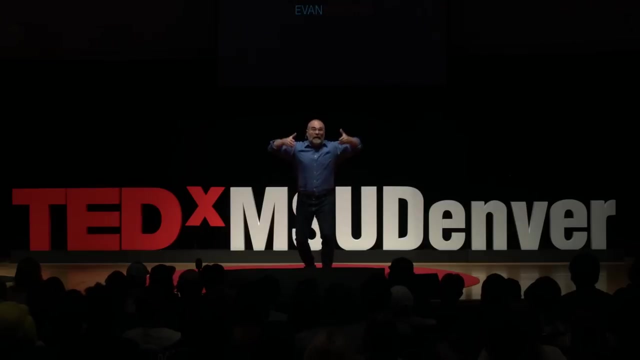 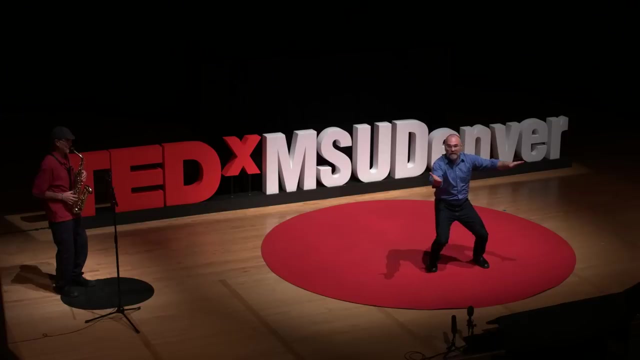 And the longer I hold this, the longer I want you to expand your awareness to the entire room and maybe, just maybe, we might discover one sound that we'll create together. So synchronize, sustain and hit You guys ready ¶¶.